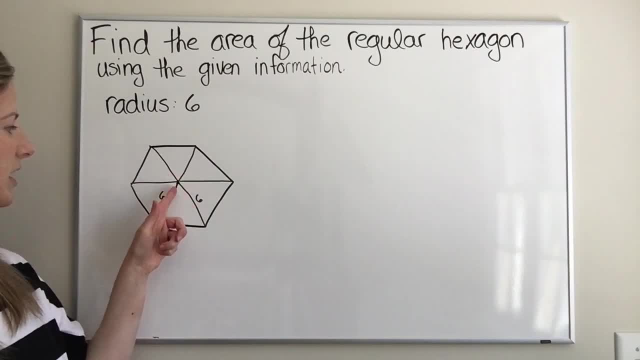 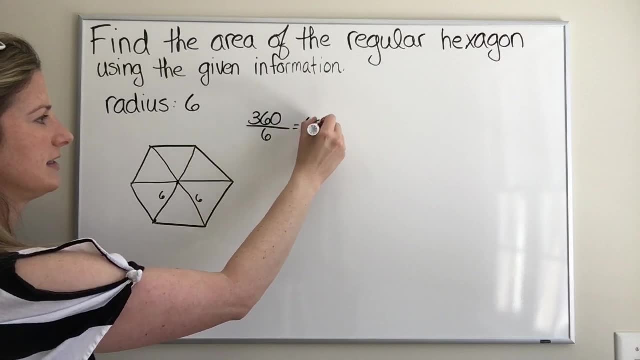 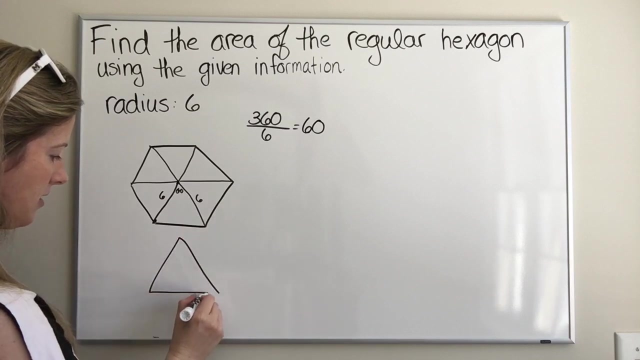 from the previous video that we are able to find this angle here by just taking 360 and dividing by the number of angles that we have. In this case, it's 6, and that's 60. So we know that this angle is 60. Okay, so if I redraw this, okay, all right, I know that this is 60 if I'm dropping. 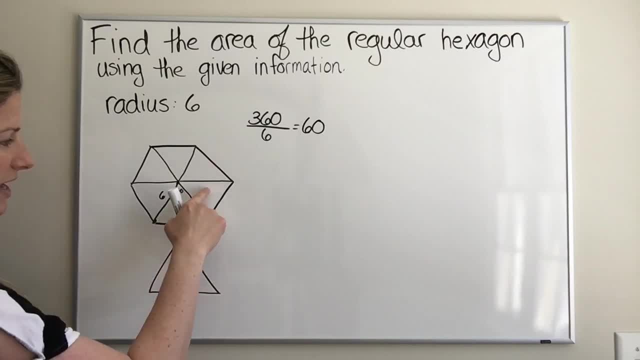 an altitude, because the whole point is I want to find the height, because if I find the area of one of these triangles, I can just multiply it by 6 to get the area of the entire polygon, the entire hexagon in this case. So this is 60, so this will go to 30.. Okay, this was 6 here, All right, so. 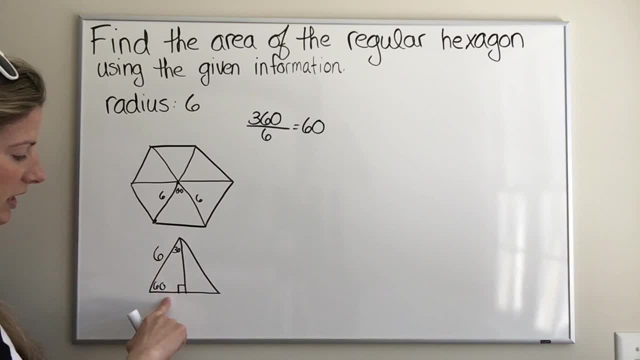 because this is a special right triangle. I'm just going to go from the hypotenuse to the short leg, which is just the short leg is half the length of the hypotenuse, and then from the short leg I can go to the long leg, which, in this case, 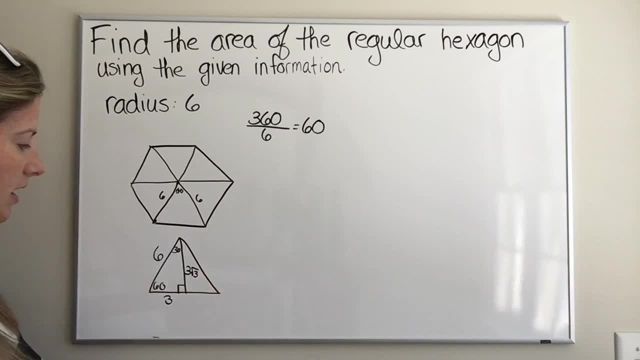 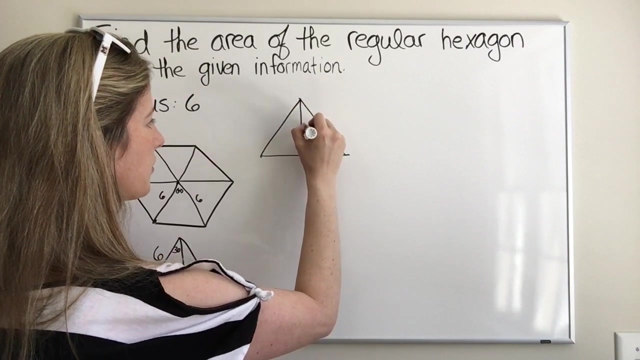 is the height, which I just multiply by root 3.. Okay, so now I am looking at a triangle, and I'll erase this right here. Now I'm looking at a triangle that has a height of 3, root 3, and a base it's going to be 6.. And the reason I know it's 6 is for two reasons. 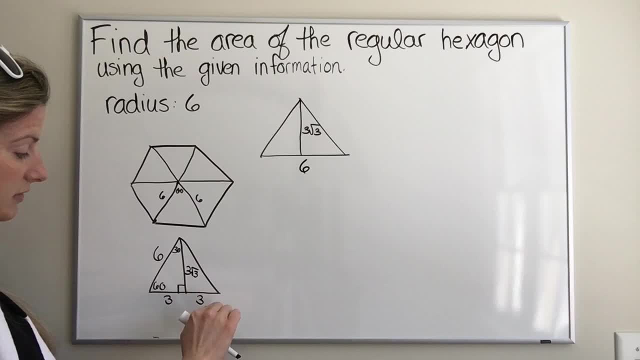 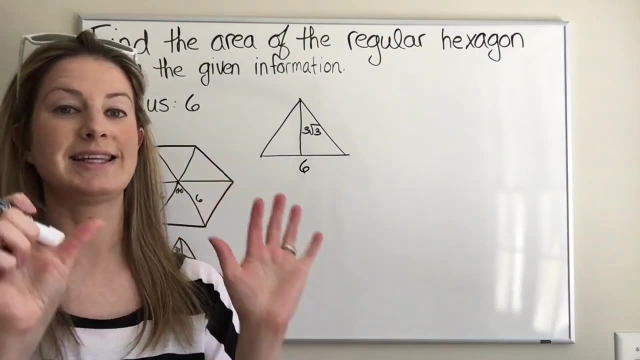 Number one. this is 3, so this is also 3, so together it becomes 6.. Or it's a unique situation with a regular hexagon where you actually create 6 equilateral triangles. Okay, so they're all 60,. 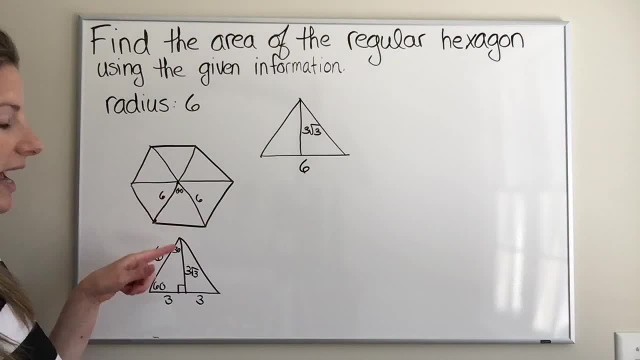 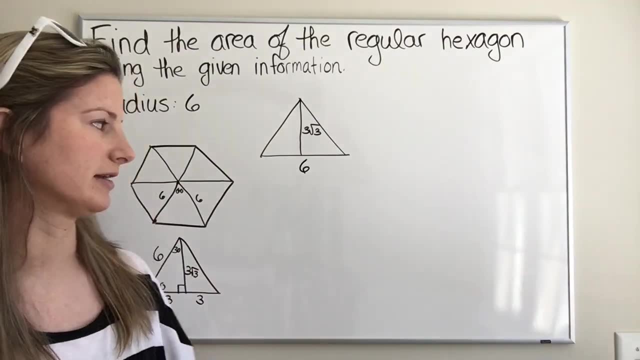 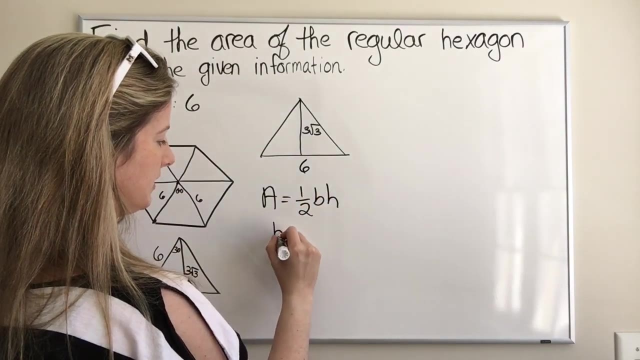 60, 60.. Okay, which means that the side lengths are all the same. The radius is the same length as the side. Okay, and that's unique to hexagons. Okay, so now, if I want the area, it's just going to be 1 half base times height. In this case, the base is 6, and the height is 3 root 3..